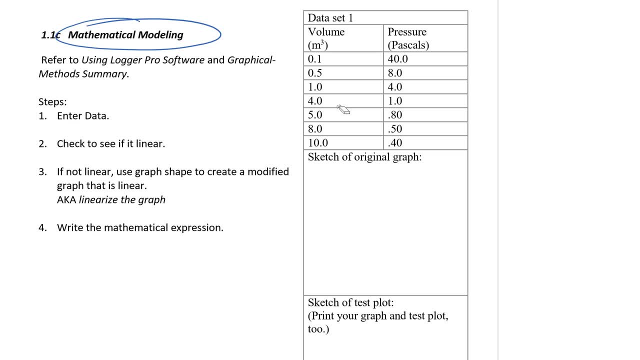 to make a mathematical model of this data. To do this you're going to need first of all it says here: refer to user using Logger Pro software. so that should be handout that you have, and also the graphical method summary should be a handout that you have. The other thing that you'll need is a. 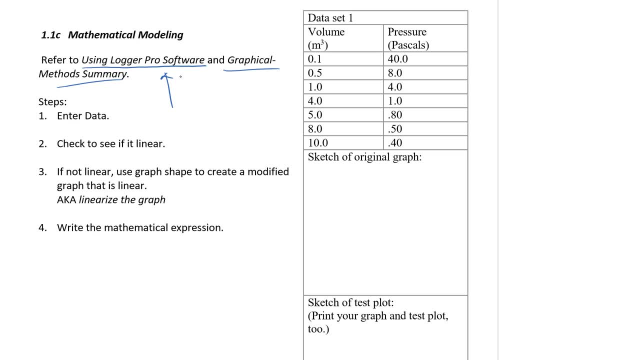 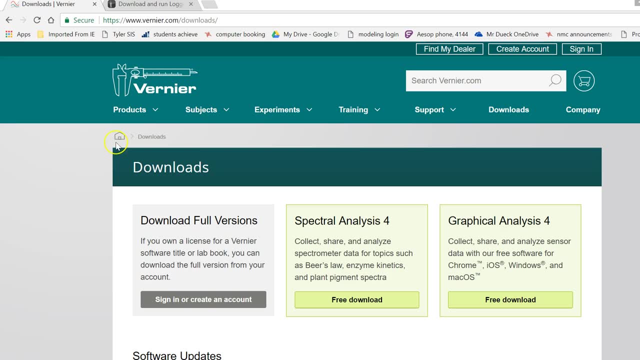 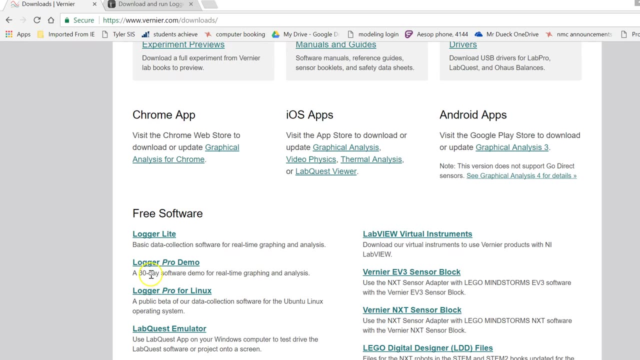 working copy of the Logger Pro So you can be using one of the school's computers- it has Logger Pro installed in it. or if you go to verniercom slash downloads you can see that up top and then you can get a 30-day- I think here it is Logger Pro demo or 30-day software demo for. 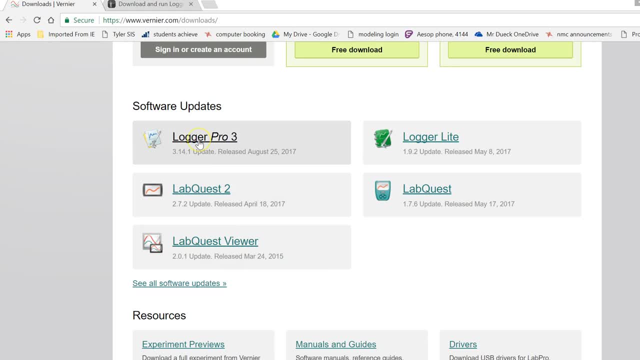 real time. so you can do that. or perhaps I'll be able to get you a license for home use. I'm not quite sure about that, but you can ask me that in class. So in either case, you'll need to have Logger Pro running right now. Here's what Logger Pro looks like. 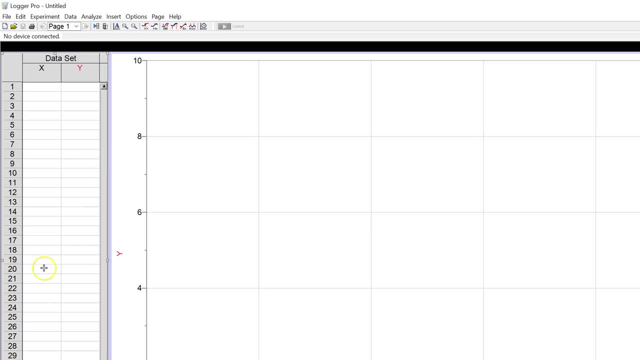 And you'll see. I can't quite put the whole screen in right now, but I'll move around with my screen capture part so you'll see stuff. So right now none of the data is in where the X and the Y is. so what we'll need to do is, step one is to take the data from that data table, that volume and the pressure. 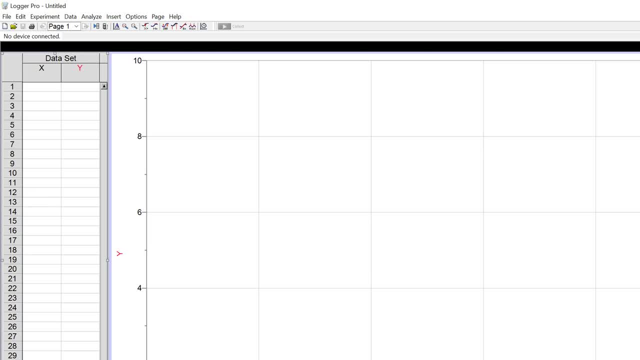 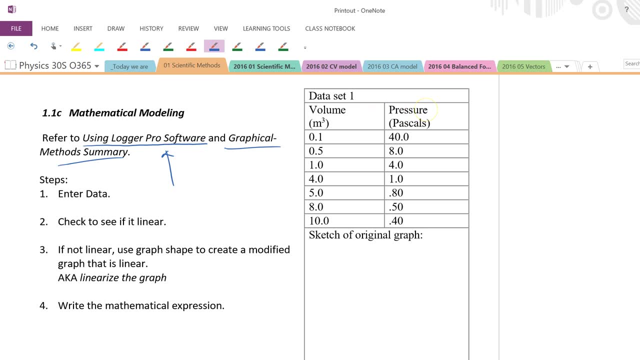 and put it in there. So if I just switch over here this, they've got volume in one column and pressure in the other column. make the assumption here that this, this first one, is going to be your independent variable and this one is going to be your depending variable. and just a reminder that when you 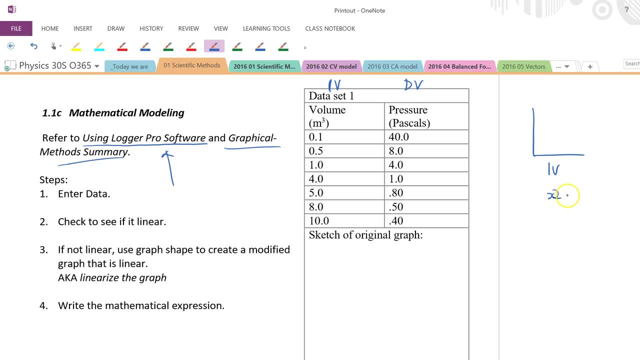 are graphing. your independent variable is what we normally use, is for the x, and your depending variable is normally what we'd use for the y. So in other words, it's kind of like what you would expect where this is the x and this is the y. So when you see the data table, you can just take this. 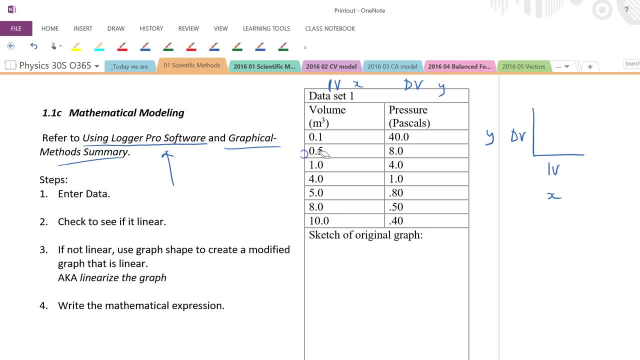 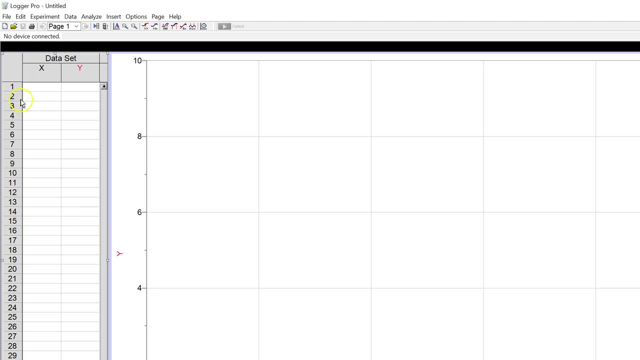 stuff and throw it in like the left hand column goes in the left hand column. So first of all we got to establish that the x is actually volume. now. So, if I go back to Logger Pro, the easiest way is just to double click on this x and then we can type this stuff in. So we put volume in here. 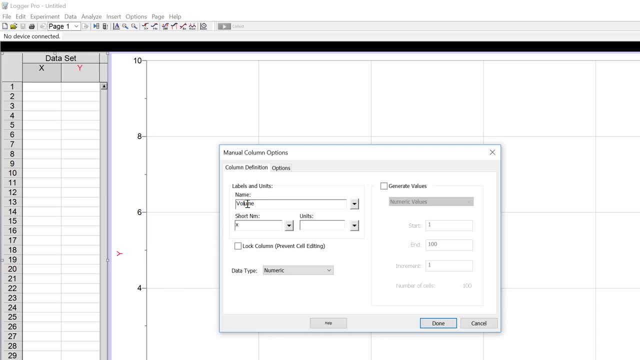 and for the short form- if I can spell that better, the short form- for that I can just put capital v and the units are going to be meters cubed. So put an m and if you'll notice, you do the s drop down arrow and you can pick the superscript 3 and then we get meters cubed. Isn't that kind of? 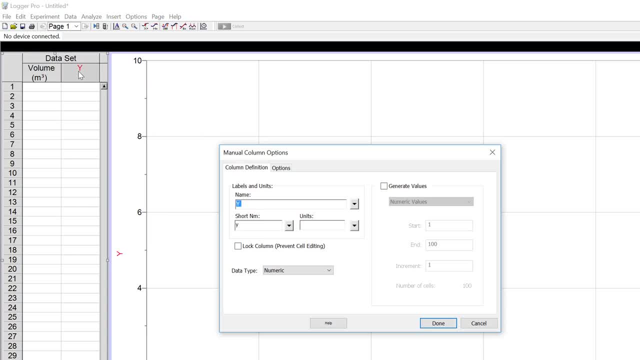 cool. And for our y we want to have pressure, So I'm going to type out pressure. The short name for that is p, and the units are pascals, which is the metric unit for pressure. I'm just going to go pa, so it's not quite as long. That's usually how we abbreviate pascals, So put that in. 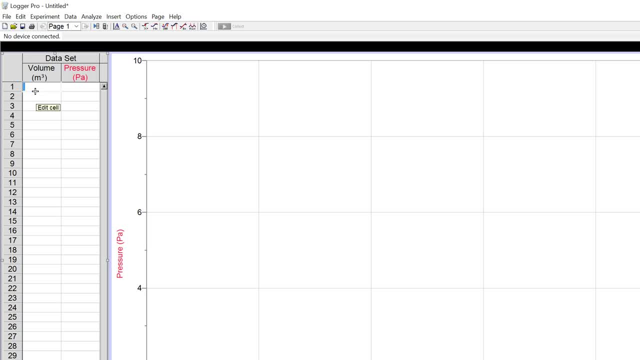 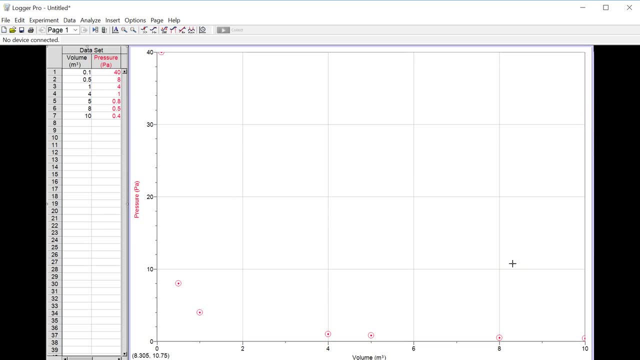 there. So you got that, and then we want to put in all this data here, So I'll just put it in There. we go, we have that all In there. I'll just resize so we can see things a bit better And you can see. now here's the top. 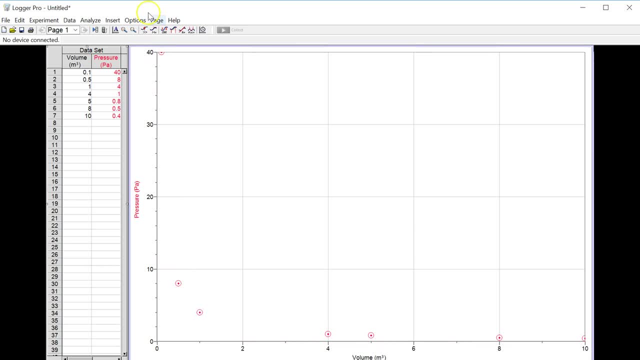 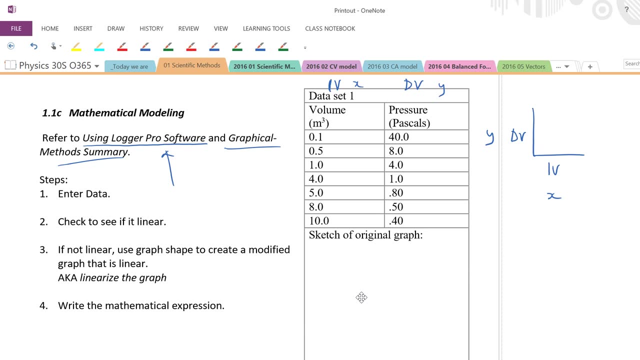 part. It's in red, It comes down and looks like this, So it kind of looks like a curve. Well, if I go and say, okay, we want to put a sketch of the original graph, So the one that we had just right now, So sketch doesn't mean, you know, doesn't have to be perfect, So I'll just put that there. 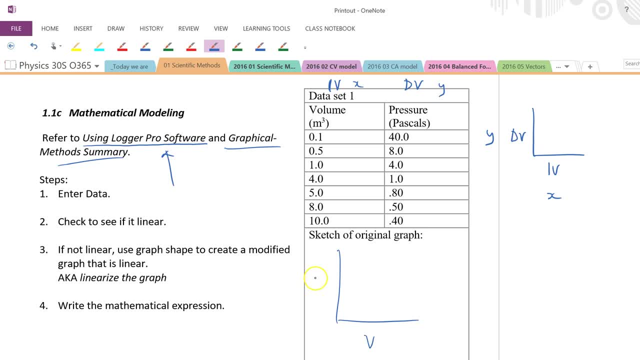 and I've got my volume here and my pressure here. How does it look? Well, it kind of has this shape over there. Okay, that's the the shape, And I know I can't draw that well because I got my keyboard out on here. So, looking at our steps: Enter data. 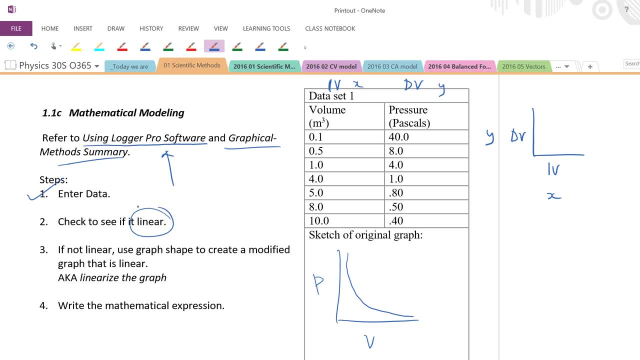 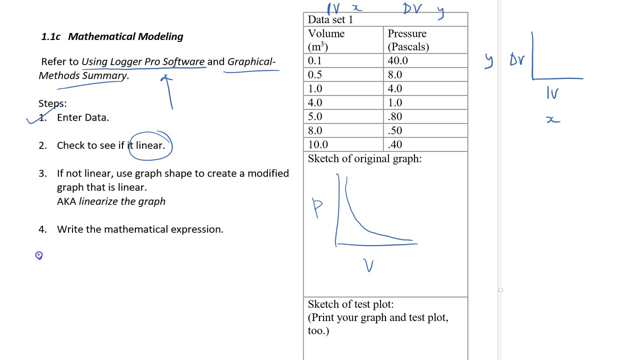 Check. Check to see if linear. What does linear mean? Linear means a straight line. Was that a straight line? No, it's not a straight line. Why do we want a straight line? Well, I'm going to say that it's actually. well, it's a straight line. Linear means интерступ. So that's a straight line. Then I'm going to hit back over here. So I want to do like this all the time here. You don't want to calculate? Then what I'm going to do is I'm going to change the constant You could do, and then something about it. We're just going to open up a perfect line. So I'm just going to multiply the noise. What I've done so far for the line is double the average line for that, So that works.